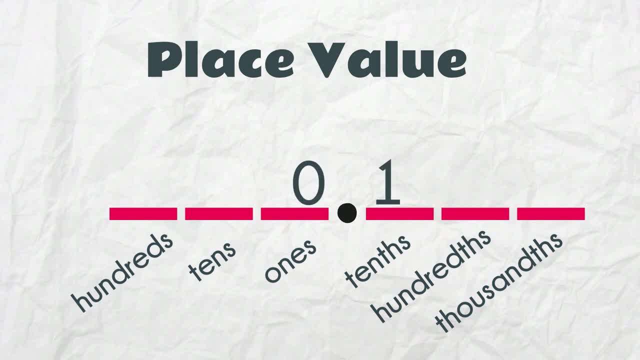 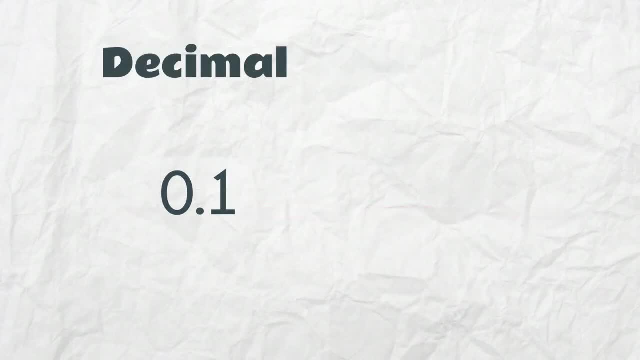 Take this decimal 0.1.. It can also be read as one tenth, because this is the tenths place. What does one tenth look like as a fraction? You guessed it: one over ten. And there's another kind of a decimal point. 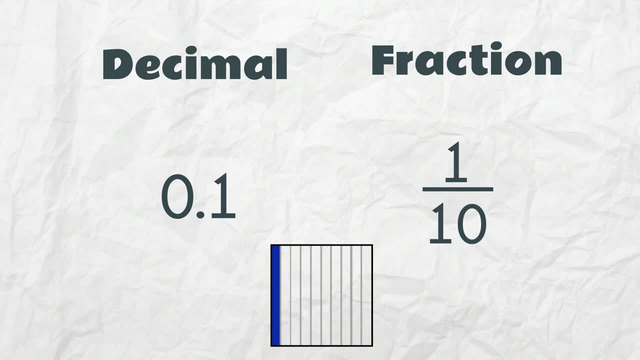 The decimal 0.1, or one tenth is the same as the fraction one tenths- They're equivalent. Here we have the two tenths's, 0.2,, three tenths, four tenths or five tenths. 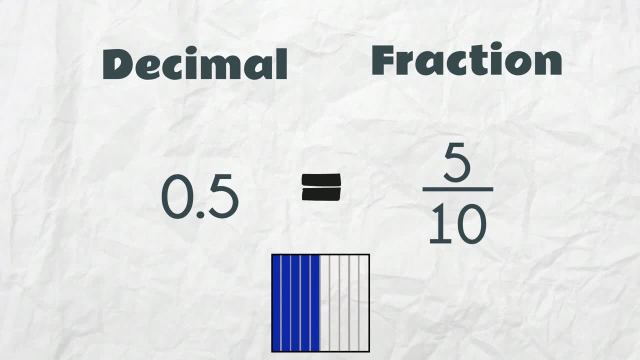 Did you notice that we can simplify this fraction? five-tenths is the same as one half. This is what you have here, And five-tenths aren't quite as simple as one impression, But if that's true, it's about the same as any fraction. 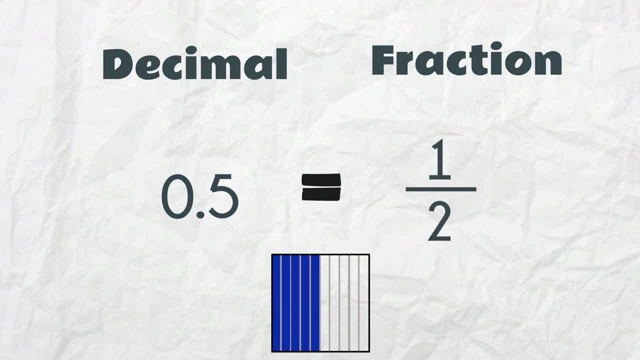 I'm going to look at fact and you're going to know some basic fractions. It's simply general hearings And I'm just going to rule Built-out, Prim, exploratory Summary clothes cheaper than enough and various avey. hmm to learn. We've probably seen one half represented as 0.5 many times before. 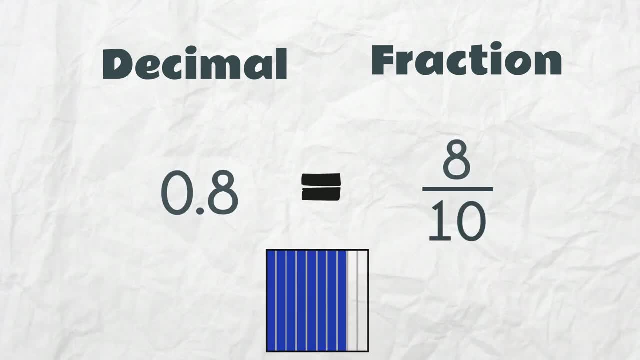 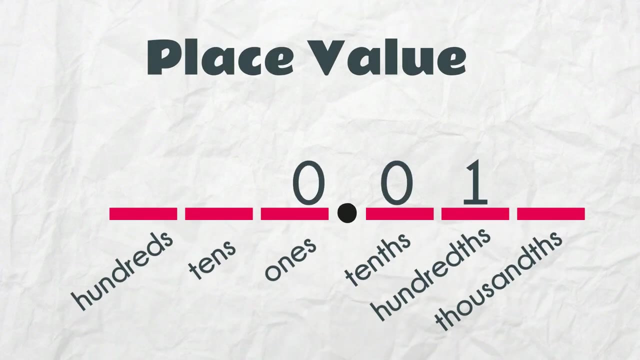 Six tenths, seven tenths, eight tenths, nine tenths. After nine tenths, we have ten tenths, which we know is just one whole. Let's move on from tenths. Look at this decimal 0.01.. 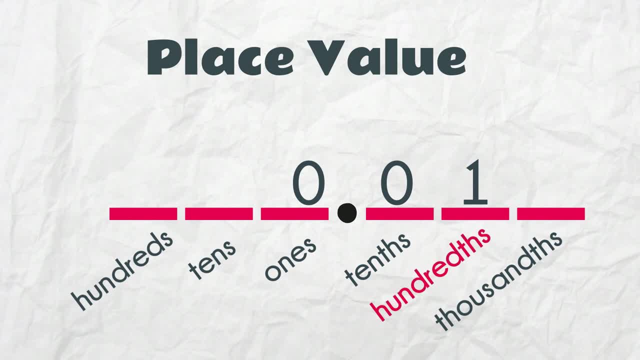 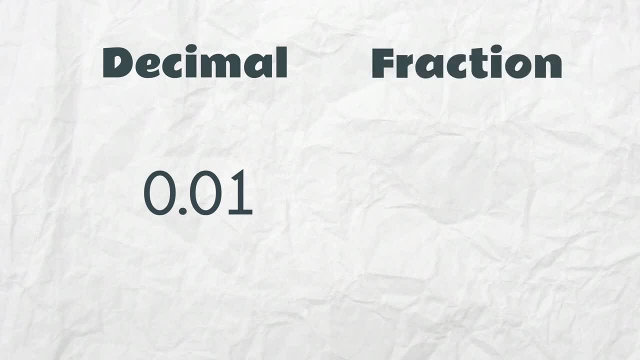 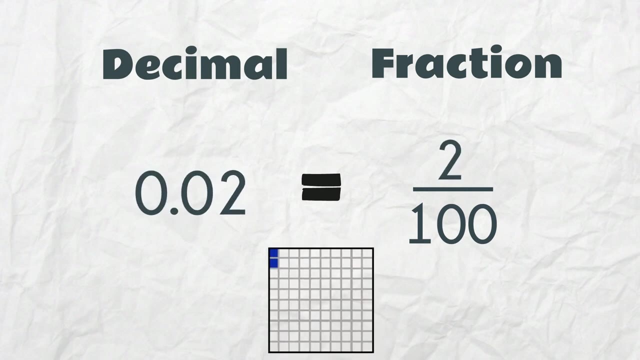 This is the hundredths place, So we can also read this decimal number as one hundredth. As a fraction, it would look like this: Two hundredths or 0.02, three hundredths, four hundredths and so on. 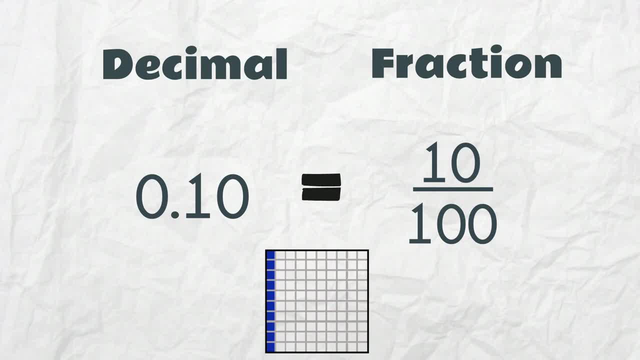 Now that we're out of time, let's look at the decimal numbers. Let's look at ten hundredths. What do you notice about the decimal form We have moved into the tenths place? Ten hundredths is the same as one tenth. 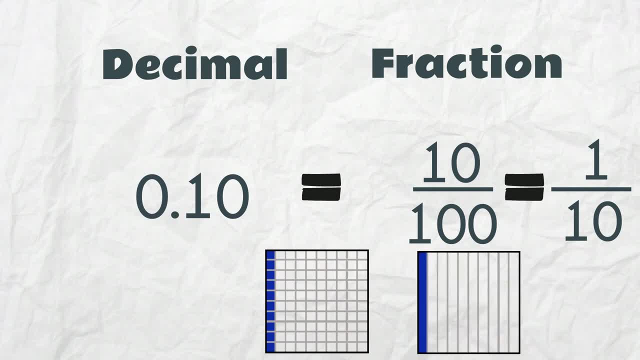 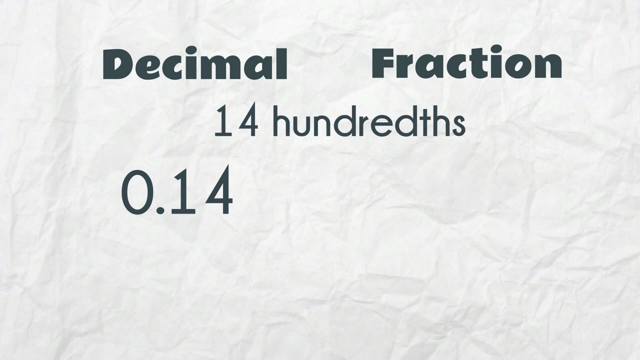 We can also see that from this model, as one tenth is overlaid on the ten hundredths, Ten hundredths is written as 0.1.. The last zero is not needed. Here we have the decimal number 0.14.. It can be read as fourteen hundredths. 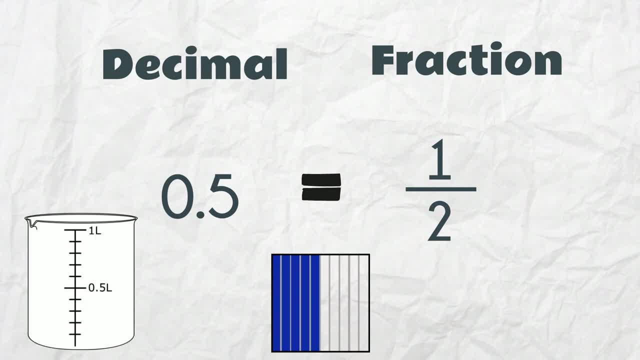 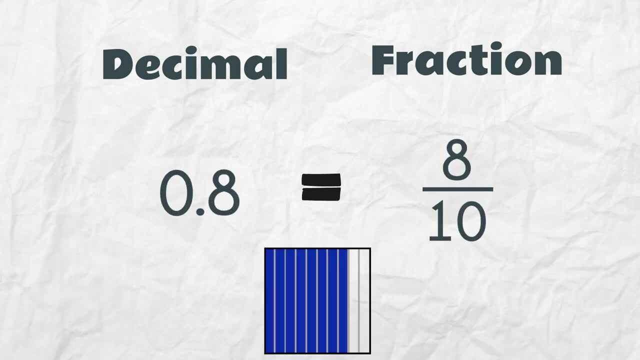 half represented as 0.5. many times before 6 tenths, 7 tenths, 8 tenths, 9 tenths. After 9 tenths we have 10 tenths, which we know is just one whole. Let's move on. 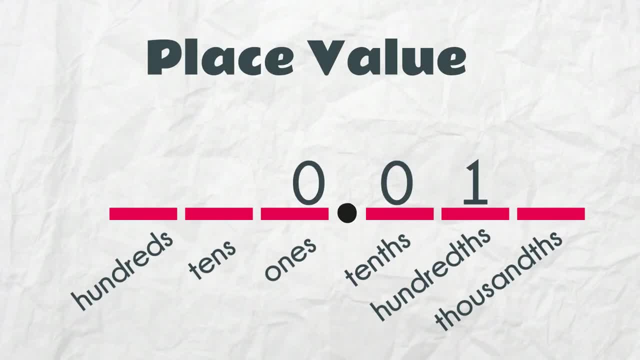 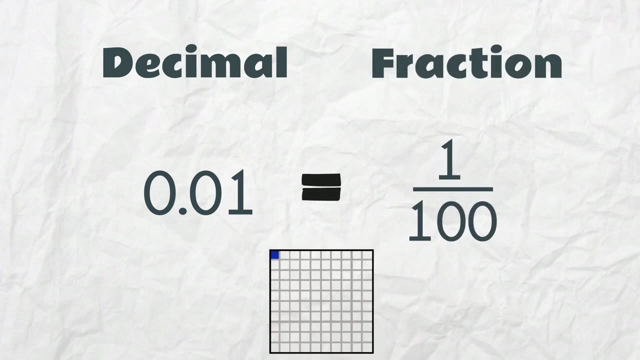 from tenths. Look at this decimal 0.01.. This is the hundredths place, so we can also read this decimal number as one hundredth. As a fraction, it would look like this: Two hundredths or 0.02, three hundredths, four hundredths and so on. 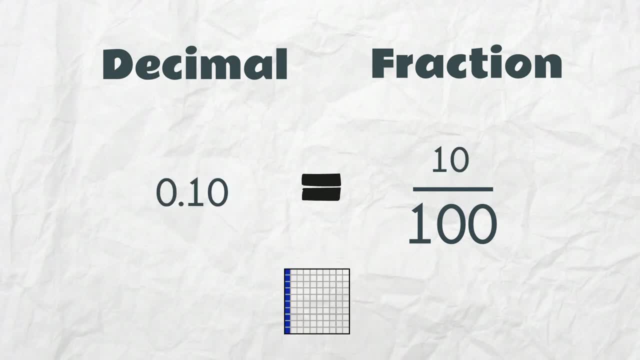 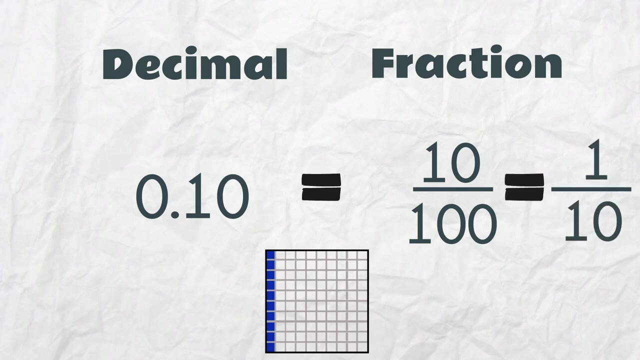 Now that we're at ten hundredths, what do you notice about the decimal form? We have moved into the tenths place? Ten hundredths is the same as one tenth. We can also see that from this model, as one tenth is overlaid on the ten hundredths. 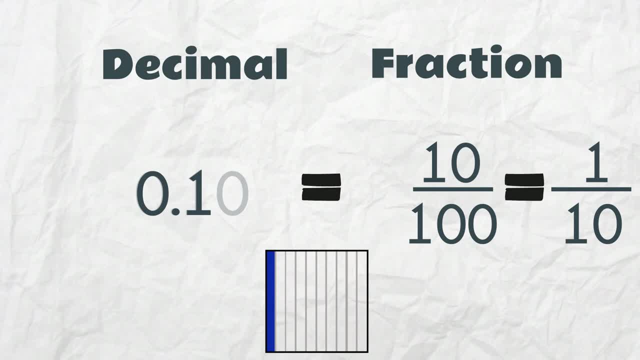 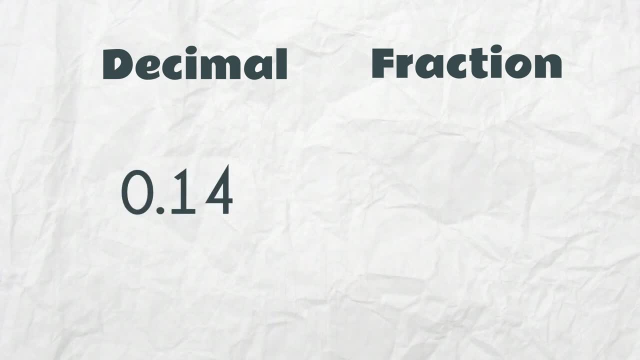 Ten hundredths is written as one tenth. Ten hundredths is written as 0.1.. The last zero is not needed. Here we have the decimal number 0.14.. It can be read as 14 hundredths. We can see that it is made up. 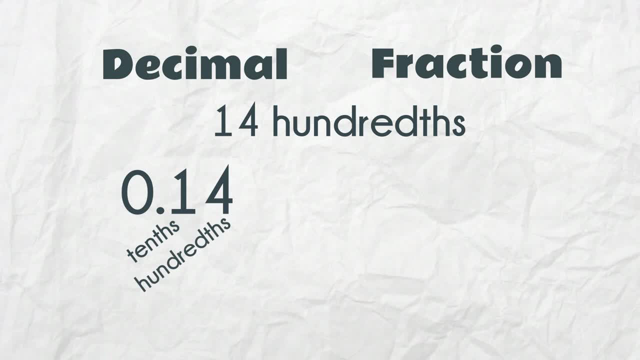 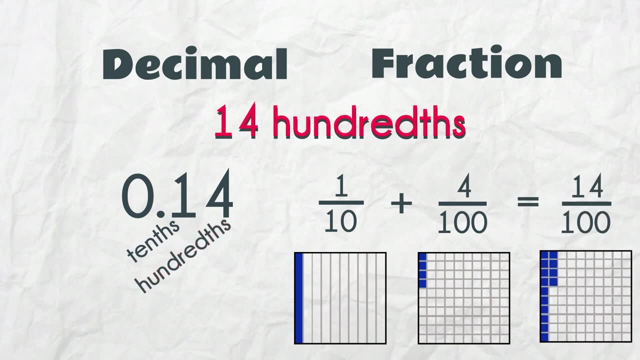 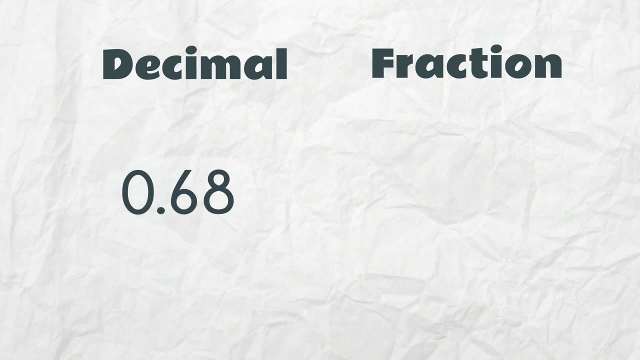 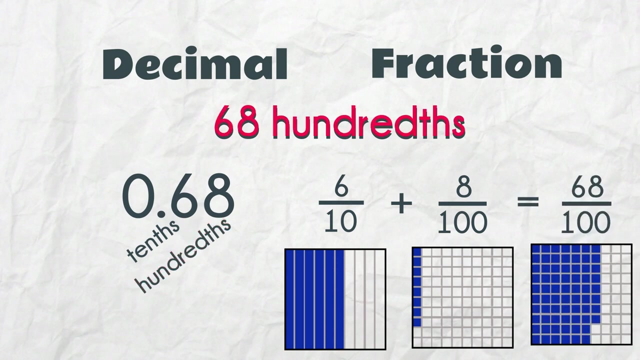 of one tenth and four hundredths. One tenth plus four hundredths equals 14 hundredths. Here is another 0.68.. It can be read as sixty eight hundredths. It has six tenths and eight hundredths. Six tenths plus eight hundredths equals sixty eight hundredths. 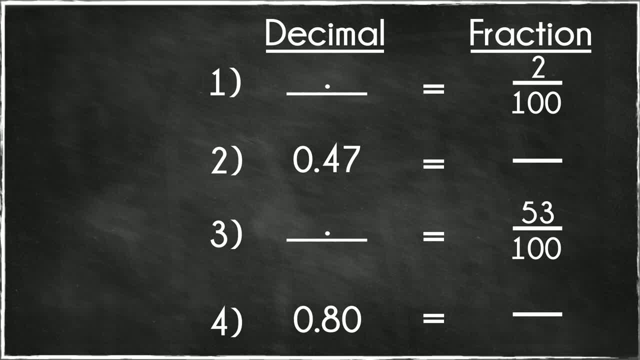 Practice converting between fractions and decimals as you complete the following table. Pause here while you work, Let's go through the answers. Number one: Two hundredths, expressed as a decimal is 0.02.. Number two: 0.47.. There are four tenths and seven hundredths. As a fraction, it is forty seven hundredths. 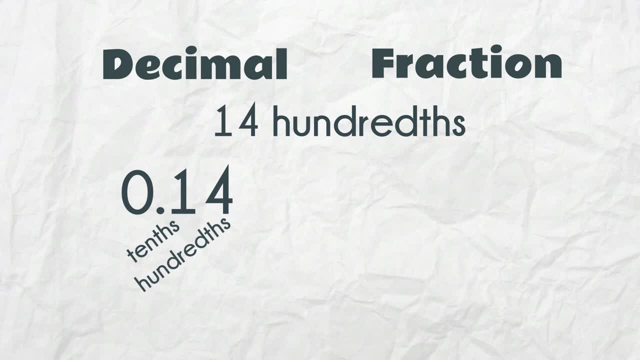 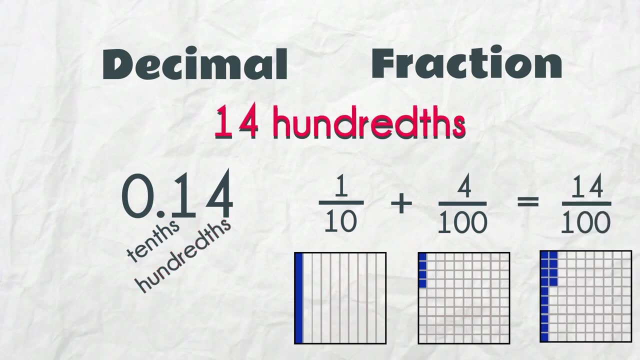 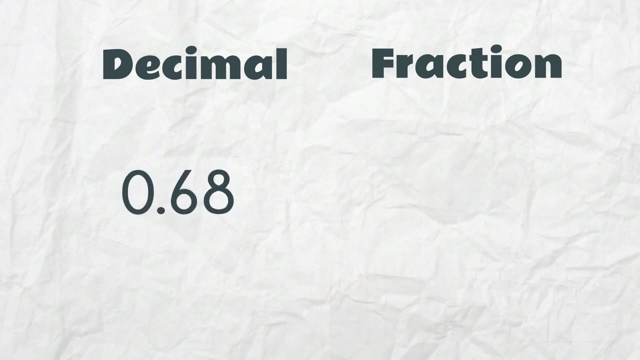 We can see that it is made up of one tenth and four hundredths. One tenth plus four hundredths equals fourteen hundredths. Here is another 0.68.. It can be read as sixty-eight hundredths. It has six tenths. 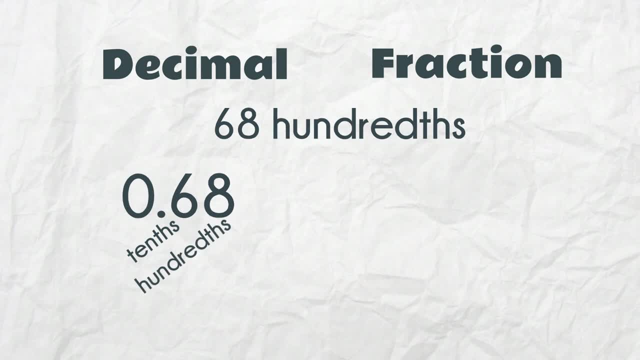 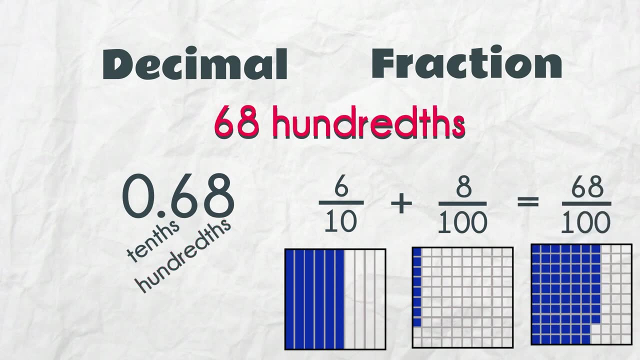 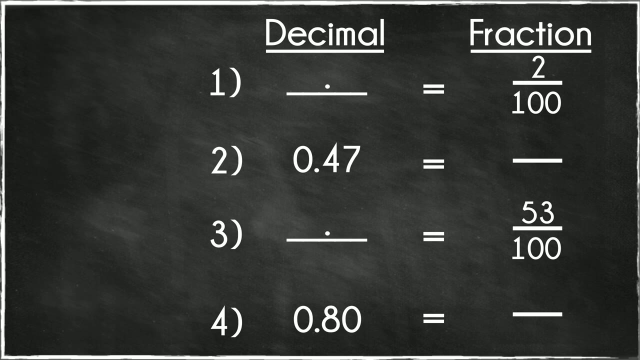 Six tenths plus eight hundredths equals sixty-eight hundredths. Six tenths plus eight hundredths equals sixty-eight hundredths. Practice converting between fractions and decimals as you complete the following table. Pause here while you work, Let's go through the answers. 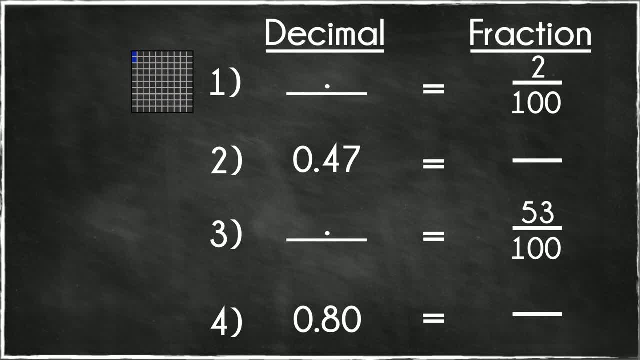 Number one: Two hundredths expressed as a decimal is zero. Number two: Two hundredths expressed as a decimal is zero. Number three: Two and a half is the decimal. The decimal is zero point zero. two Number two. 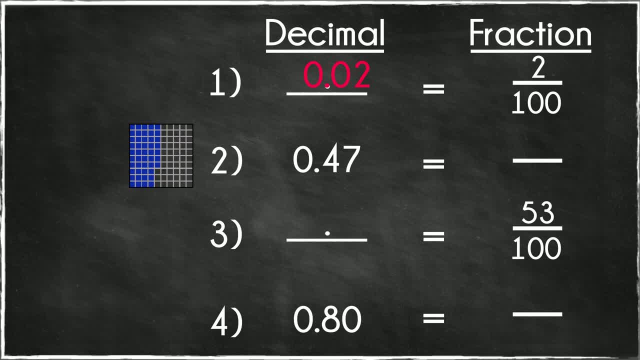 Zero point four, seven. There are four tenths and seven hundredths. As a fraction it is forty-seven hundredths Number three. Fifty-three hundredths as a decimal is zero point five, three, Number four. Did this zero throw you off? 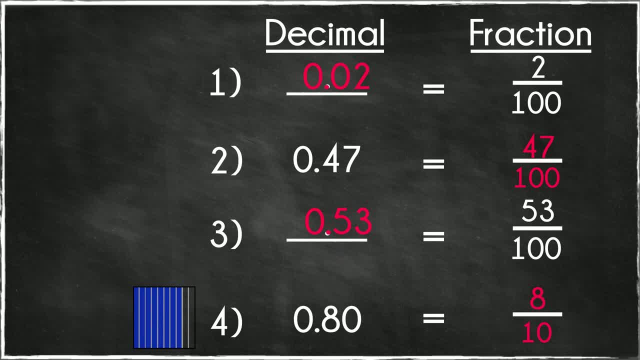 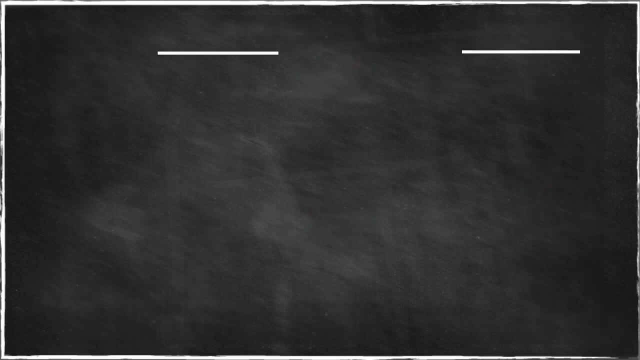 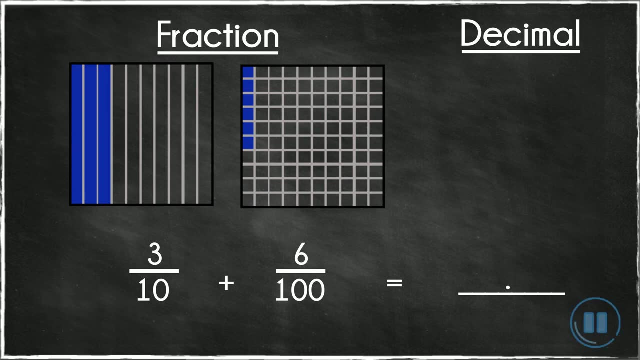 This decimal number has eight tenths, and so is written. as eight tenths might have written 80 hundredths, which is also correct. Let's try a couple more: 3 tenths plus 6 hundredths Show the answer as a decimal Pause here The. 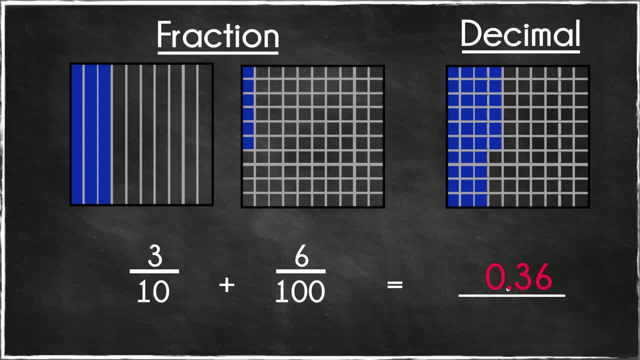 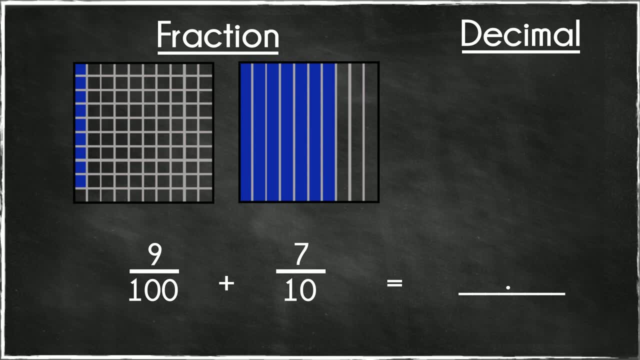 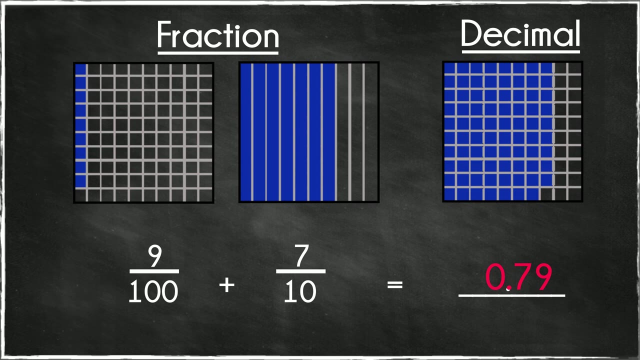 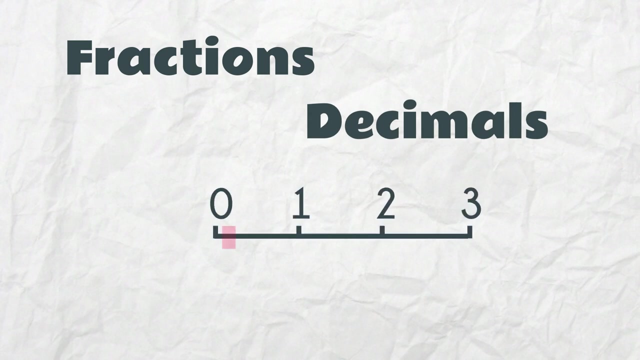 answer is 36 hundredths 0.36.. One more 9 hundredths plus 7 tenths. Show this as a decimal and be careful with this one Pause here. The answer is 79 hundredths 0.79.. Remember: fractions and decimals do the same job. They both show amounts that. 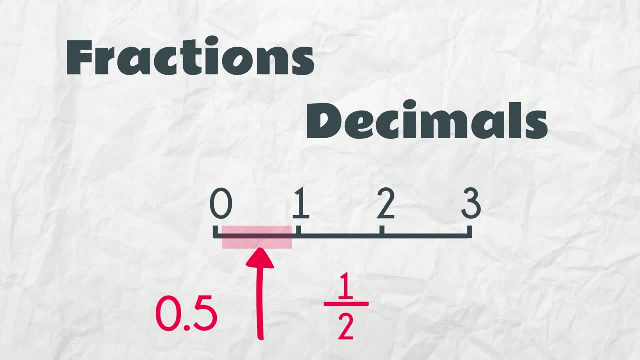 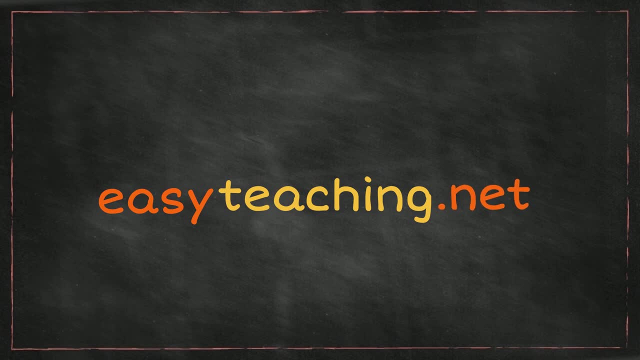 are in between whole numbers: EasyTeachingnet. wwweasyteachingnet.